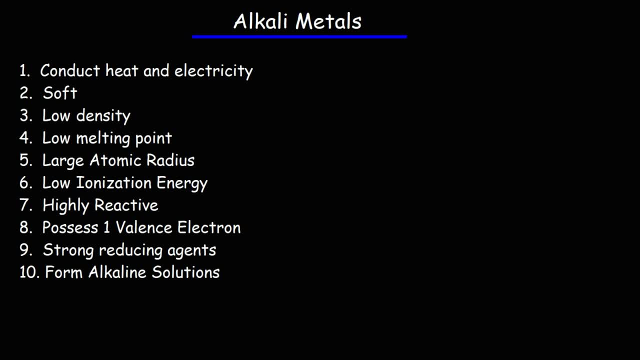 of around 29 degrees Celsius. Now they also have a large atomic radius. Atomic radius increases towards the left, So sodium is larger than magnesium. As you go to the left, the atomic radius increases. So alkali metals: they have a relatively large atomic radius for their period, That is, if you compare them with other. 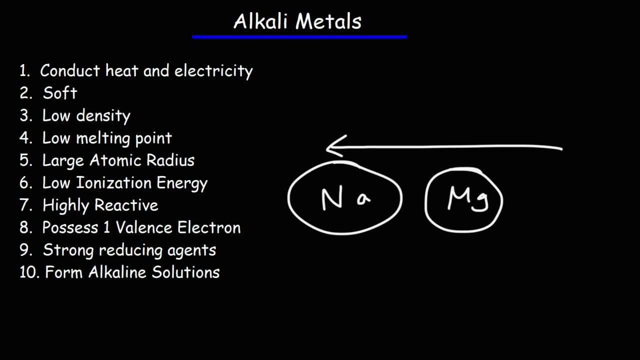 elements in the same row. Alkali metals also have a low ionization energy. Ionization energy increases to the right across the periodic table, So that means that sodium has a lower ionization energy than magnesium. Alkali metals are highly reactive. They can react with water, producing hydrogen gas and. 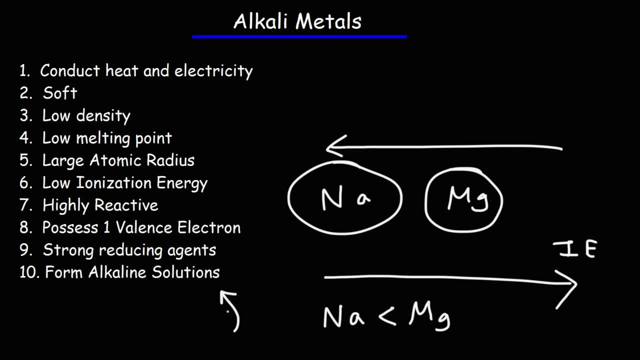 at the same time collapsing structure makeup. mo count is already there. Alkali metals have all the elements given down to the next table. They can create hydroxides so they can form alkaline solutions, All of the alkaline metals. they possess one valence: electron. 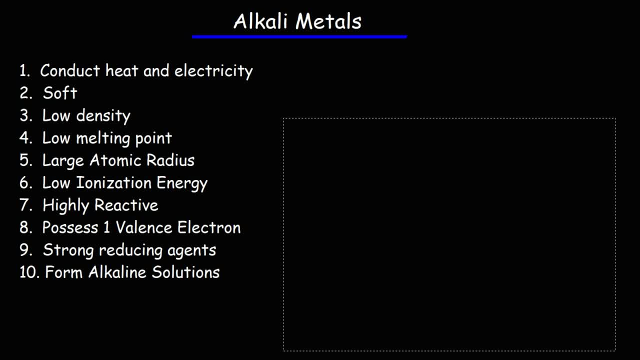 And so they have a very low electronegativity. They're, in fact, electropositive, which makes them strong reducing agents. They really want to give up their valence electrons to have a complete octet, But lithium is one of the strongest reducing agents out there. 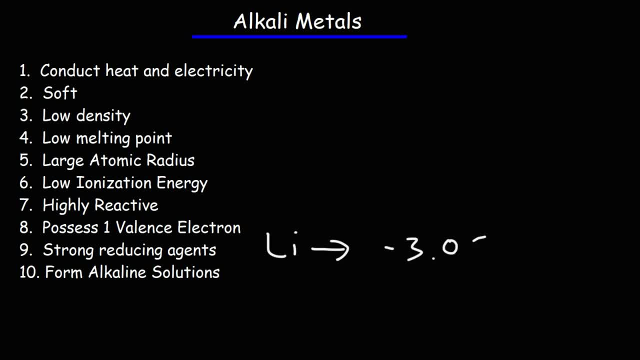 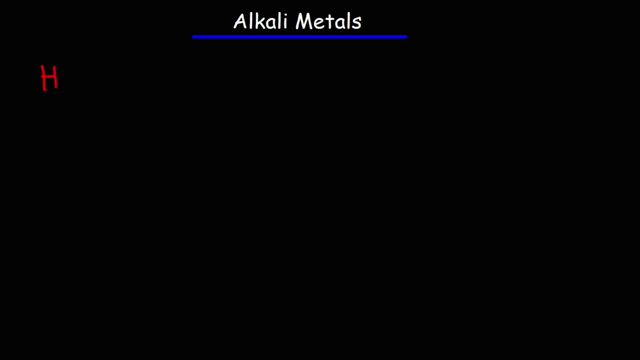 It has a standard reduction potential of negative 3.05 volts. Now let's get rid of that. So if you go to the periodic table in the first column, the first element you're going to see is hydrogen. Below hydrogen we'll have the elements lithium, sodium. 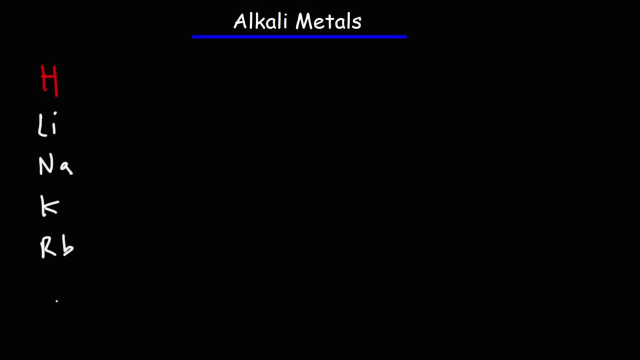 Potassium, rubidium, cesium and francium. The elements below hydrogen are considered the alkali metals. They can conduct electricity. they're soft. they have these properties. Hydrogen is considered to be a nonmetal. At room temperature, hydrogen is actually a gas. 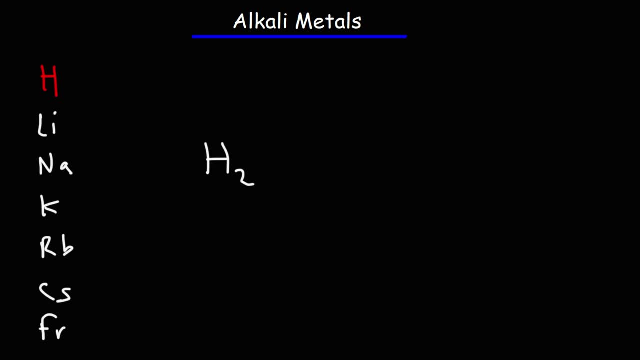 So it's not a solid metal. So, on a test, if you're asked if hydrogen is considered an alkali metal, for the most part it's not. However, hydrogen, like the other alkali metals, do contain only one valence: electron. 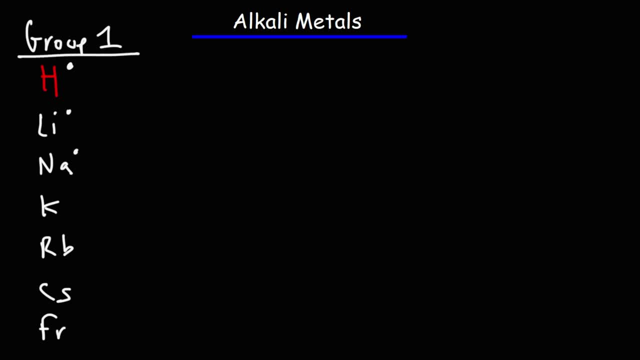 Since they're all part of group 1.. Now, as you go down this group, the reactivity of the alkali metals increases. So what this means is that francium is more reactive than cesium. Cesium is more reactive than rubidium. 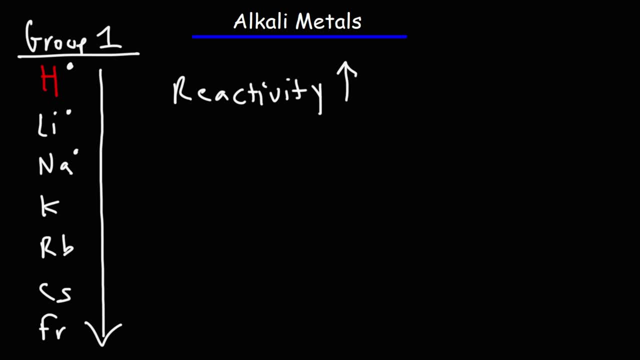 In fact, cesium reacts violently with water. Now, as you go down the group, the melting point decreases. Cesium has a very low melting point, and the same is true for francium. The boiling point also decreases as you go down the group. 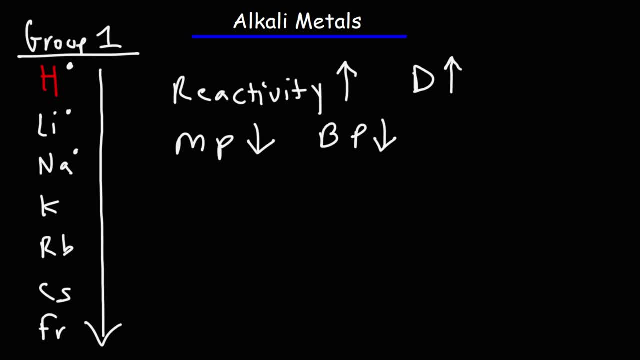 The density increases as you go down group 1. The first ionization energy, let's call it IE1, that decreases as you go down the group. The electronegativity also decreases as you go down, So lithium is more electronegative. 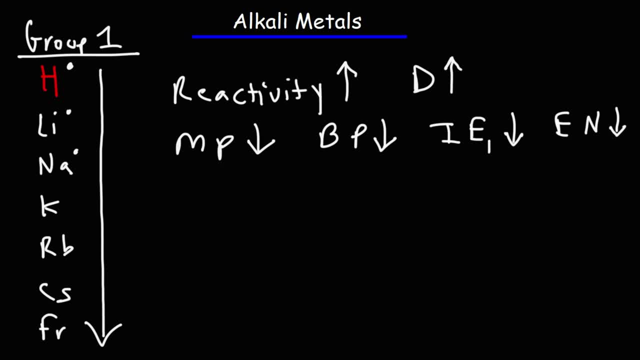 Electronegative than cesium, Which means cesium is more electropositive than lithium. The atomic radius- I'm going to put this here. The atomic radius increases as you go down, And the same is true for the ionic radius. 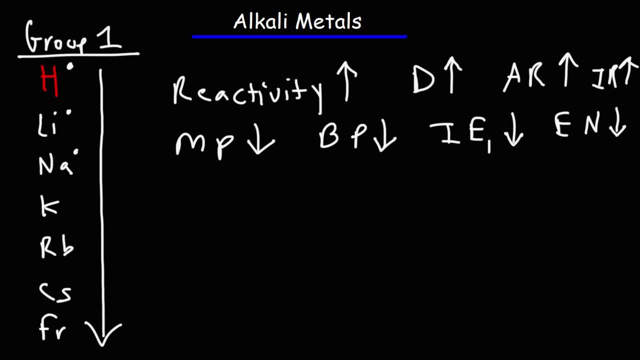 That increases as you go down the group. So those are some trends that you need to be aware of when dealing with the alkaline metals. Now let's go over some reactions with regard to the alkaline metals. 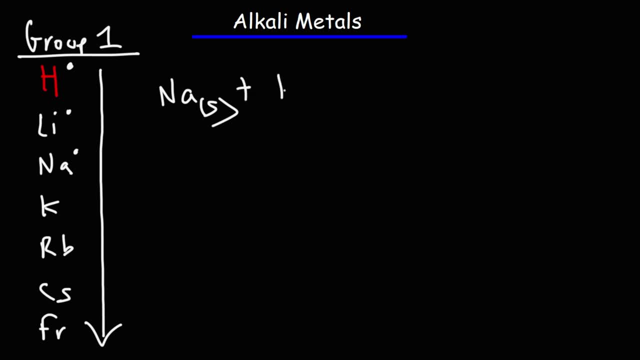 Sodium can react with water to produce an alkaline solution, Sodium. it will create sodium hydroxide and hydrogen gas. So to balance this equation we need to put a 2 in front of sodium. 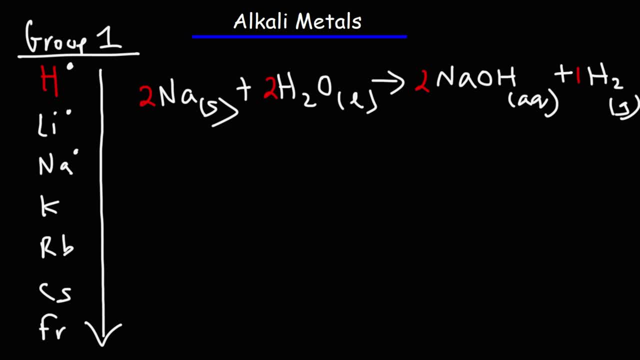 water and sodium hydroxide. Lithium can react with water the same way. It will produce lithium hydroxide and hydrogen gas. So the alkaline metals are strong reducing agents. They like to give away their electrons. 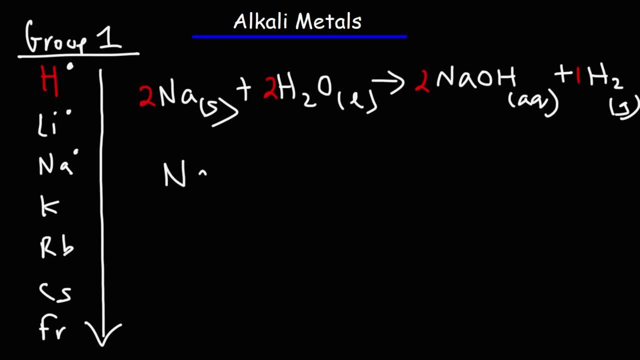 to form metal cations. When sodium gives away its electron it will form a positive metal cation And the reduction potential for that I wrote it down somewhere: it's 2.71 volts If you reverse the reaction. 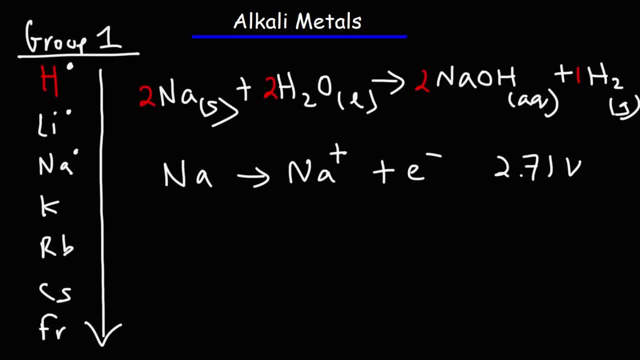 it will be negative 2.71.. That will give you the standard reduction potential. Lithium is also a strong reducing agent. The way it's written, the reduction potential here is 3.05.. If you reverse it, you get the standard reduction potential. 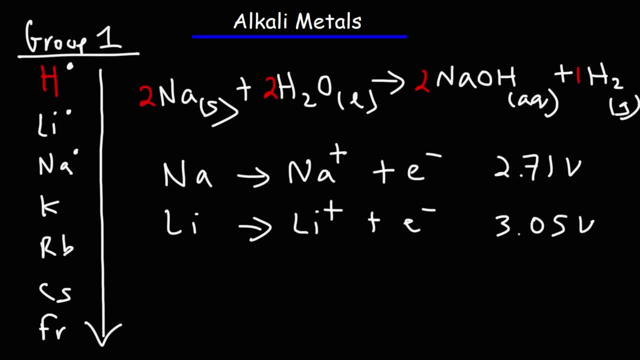 of negative 3.05.. But notice that lithium is a stronger reducing agent than sodium. It has a higher potential. Now sodium can also react with chlorine gas to produce table salt, sodium chloride. 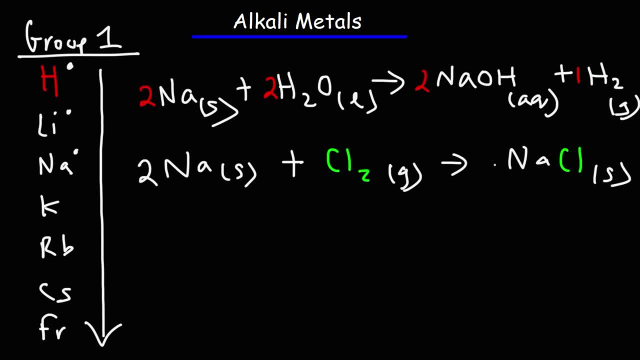 So to balance this, we need to put a 2 in front of Na and NaCl. Now the alkaline metals: in addition to reacting with water, they can also react with air. Lithium can react with. 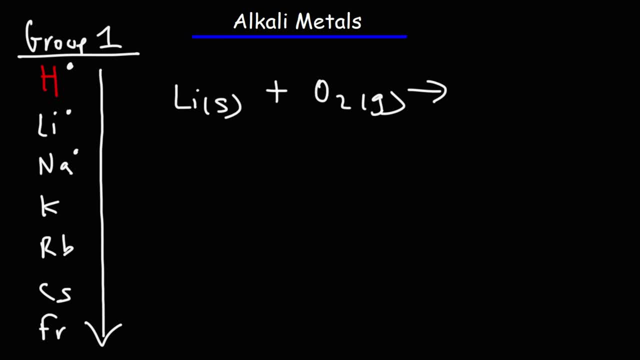 excess oxygen gas to create lithium oxide allied to O. The oxide ion is represented by this formula O with a negative 2 charge. Sodium can also react with. 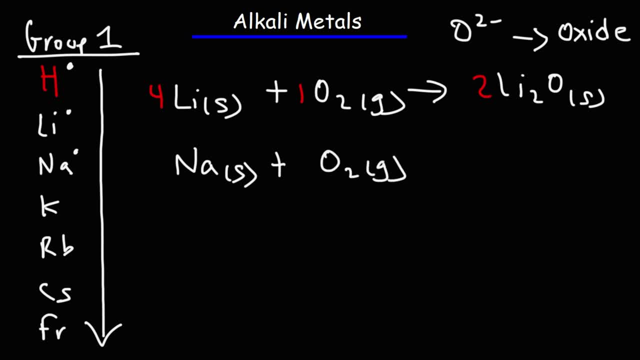 the oxygen gas in air to produce sodium oxide. Very similar to the previous reaction, But there's one slight difference here. When lithium reacts with excess oxygen, it creates lithium oxide. When sodium reacts with limited oxygen, 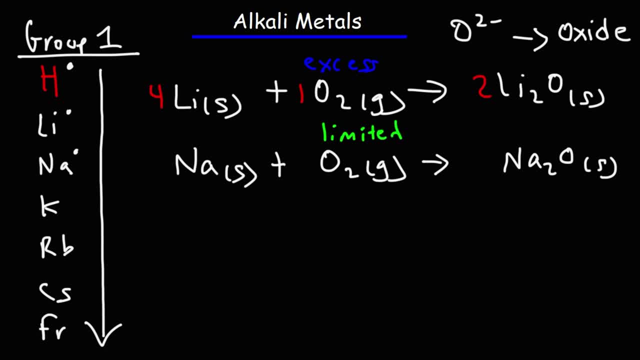 it'll create sodium oxide as well. But when sodium reacts with excess oxygen gas, we're going to get a different product. We're not going to get sodium oxide, We're going to get sodium. 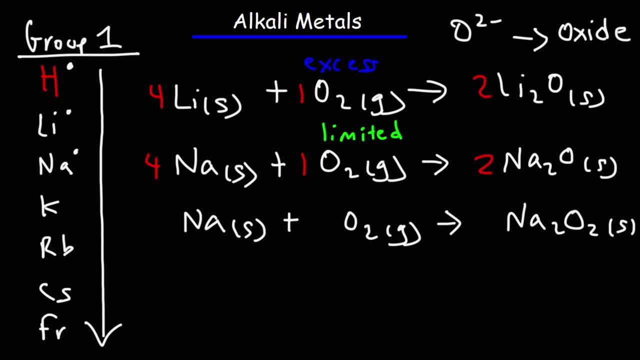 peroxide. So to balance this, all we need is a 2.. in front of sodium Per oxide has this formula: It's O2 2-. Now if we take potassium and react it with oxygen gas, 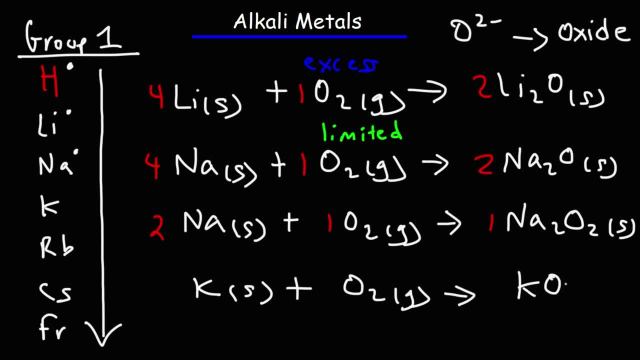 we're going to get potassium superoxide. So superoxide is O2. with a negative 1 charge, Whereas peroxide is O2 with a 2- charge. So keep that in mind If you react sodium. 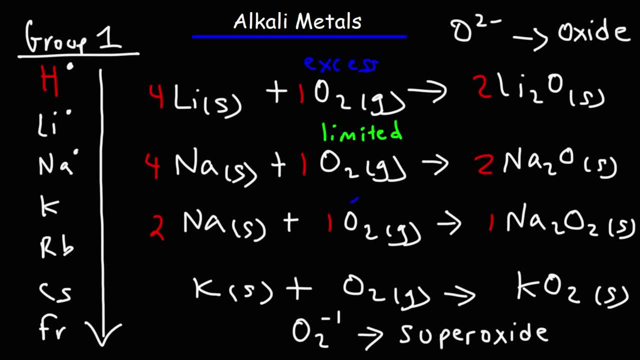 with limited oxygen you get sodium oxide. But with excess oxygen you get sodium peroxide. But when you react potassium with oxygen, you get super potassium superoxide. So those are some of the reactions that you might be. 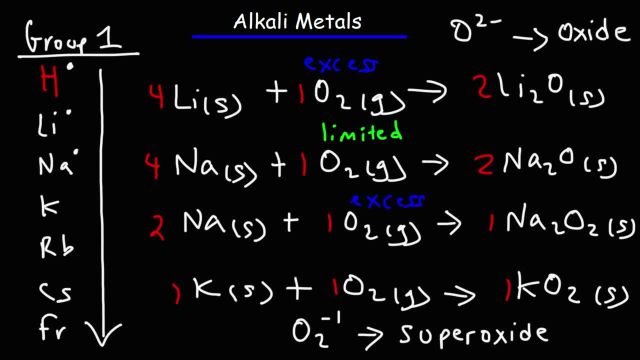 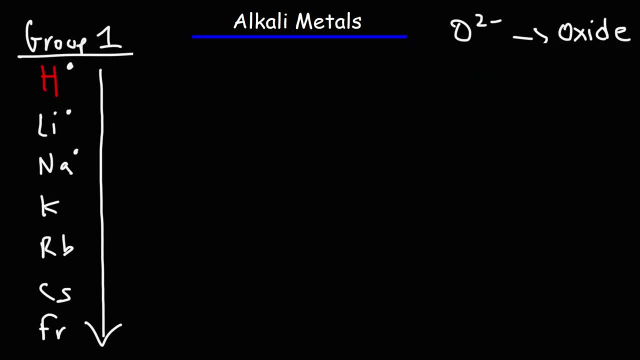 tested on with regard to alkaline metals. Now let's talk about the reactivity of alkaline metals. The reactivity increases as you go down the group. So what that means is that cesium. 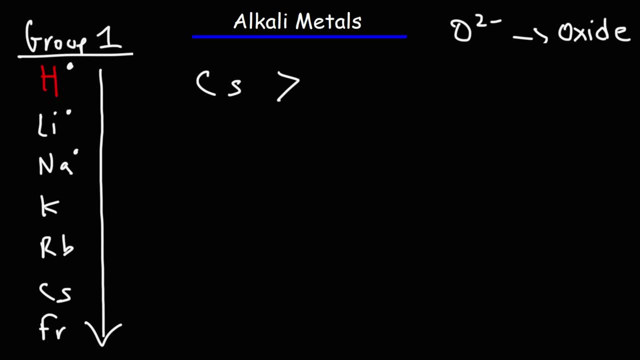 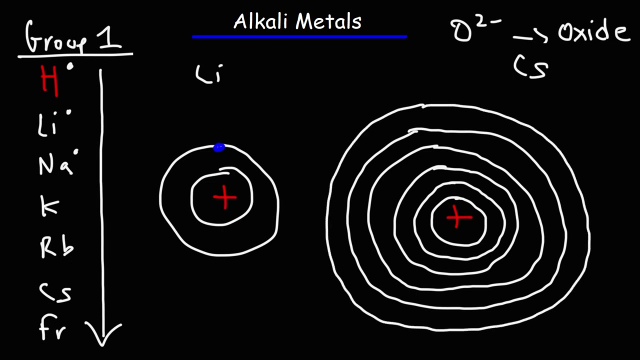 is more reactive than lithium. Now let's understand why So lithium? fourth, fifth and here is the sixth one, We can see why cesium can give up its valence electron a lot easier than lithium. 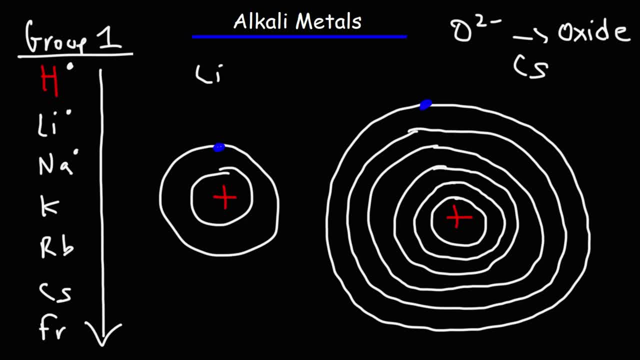 One reason for that is that this electron is very far away from the nucleus and so the pull that the nucleus have on this electron it's a lot weaker since they're further away. In the case of lithium, the nucleus has a stronger pull on the valence electron because it's so close. 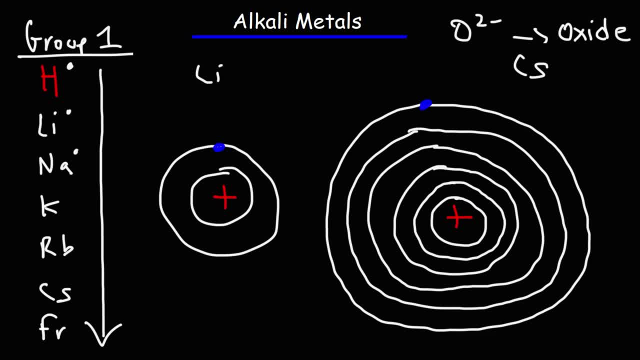 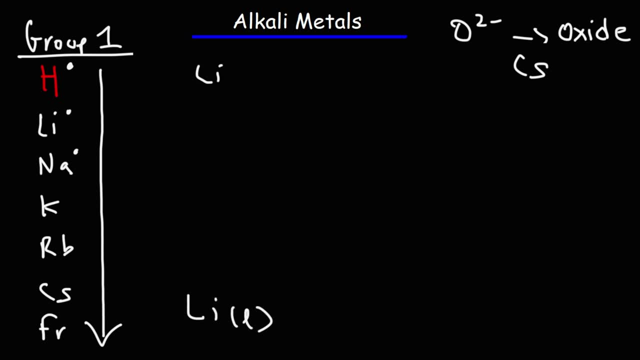 So that's one reason why cesium is much more reactive than lithium. Another reason, in fact a more important reason, has to do with the melting points of these two metals. Molten lithium is much more reactive than solid lithium because in a molten state there's 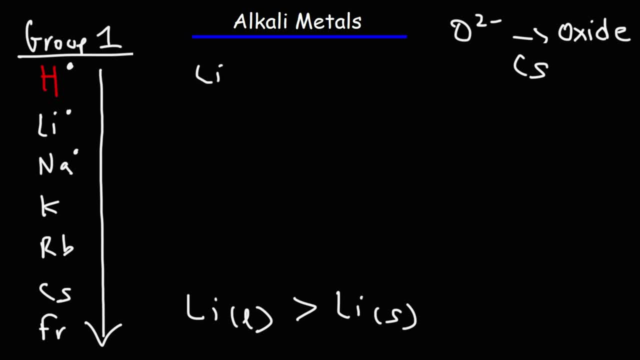 more surface area for the molecules to react, or rather for the atoms to react. Lithium has a much higher melting point than cesium. The melting point for lithium is about 180 degrees celsius. The melting point for cesium is around 29 degrees celsius. 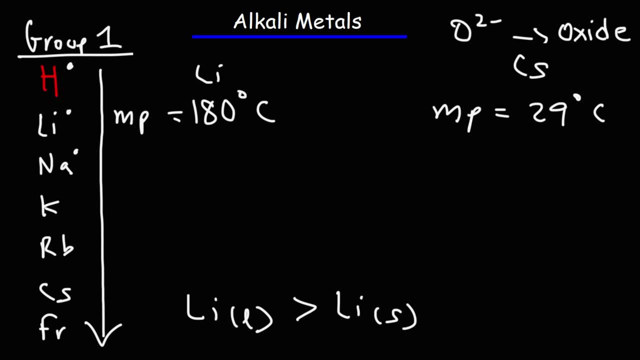 Both of these alkali metals can react vigorously with water. In fact, they're exothermic. They generate a lot of heat. Lithium, because it has a higher melting point, it's going to take a longer time for it to melt. Cesium is going to enter the molten state a. 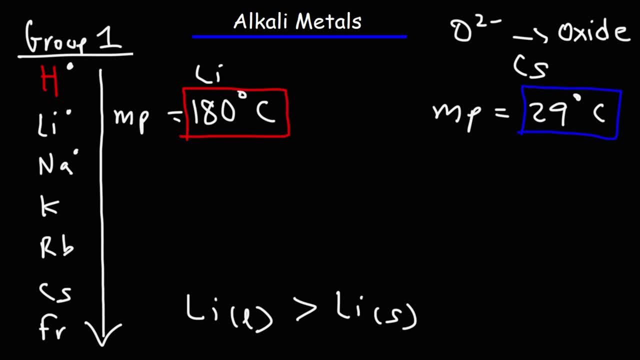 lot faster. Lithium is going to take a longer time for it to melt. Cesium is going to enter the molten state a lot faster Then lithium, because the melting point is so much more. It's so much lower. As a result, when it enters the molten state, it's going to have a greater surface area. So there's 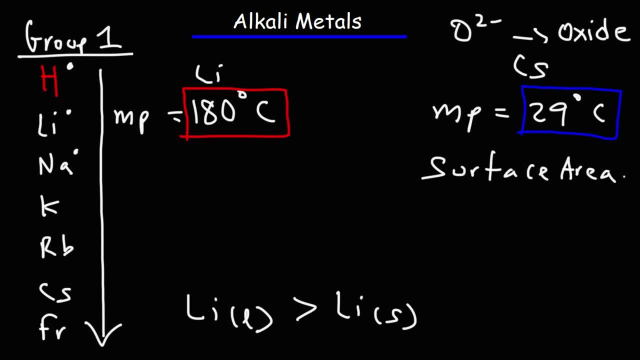 going to be more contact between the atoms of cesium and the water molecules. So with that increased surface area leads to an increased reaction rate And as the reaction proceeds faster it's going to generate even more heat, which will further accelerate the rate of reaction. 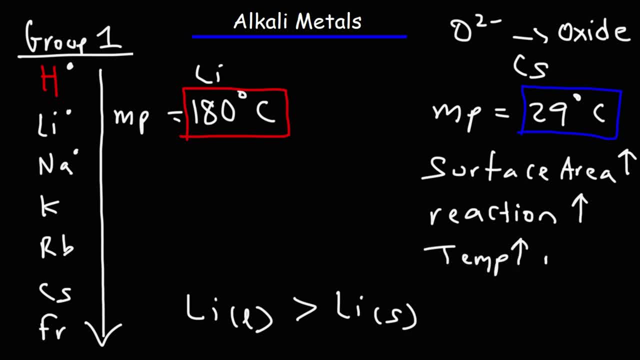 Because when the temperature goes up, the rate of the reaction goes up as well, And so all of these factors will increase the rate at which cesium reacts with water, But primarily it's due to the fact that it has a low molten point. 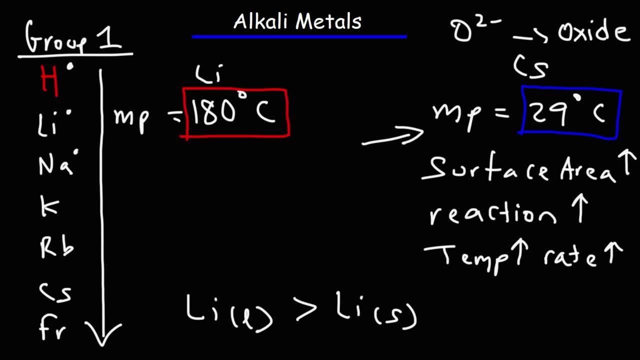 and so it can enter the molten state faster, And that's why it can react faster. Metals in a molten state will react faster than metals in a solid state. Now the standard reduction potential for lithium we mentioned. it was negative 3.05 volts. 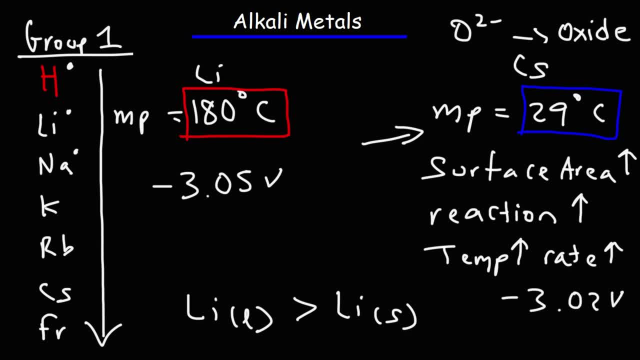 For cesium it's negative 3.02 volts. So even though lithium is a stronger reducing agent than cesium, because cesium is bigger and because it has a lower melting point, it turns out that cesium reacts with water a lot faster. 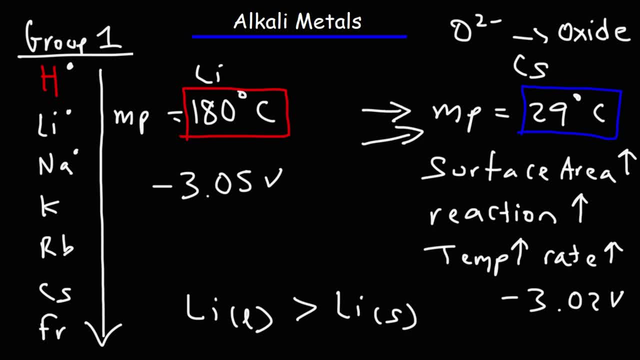 But a big reason is due to the fact that it has a low melting point, and so it can. it can quickly enter the molten state, Thus increasing the surface area, increasing the rate of the reaction, and as the reaction proceeds faster, more heat is generated. 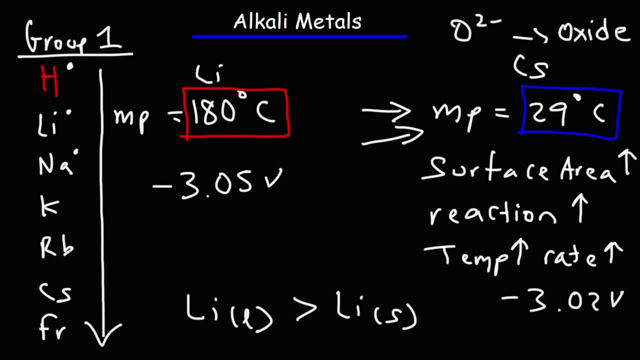 the temperature goes up rapidly, which also further accelerates the rate at which the reaction proceeds. So what you need to know is that as you go down the group, the melting point decreases, and so the reactivity of the alkaline metals will increase. 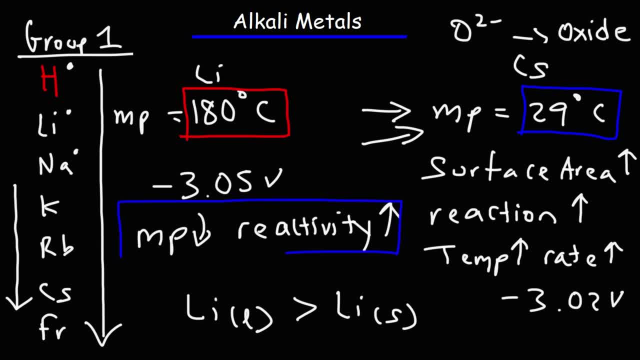 So that's basically it for this video. Hopefully it gave you a good introduction into the properties of alkaline metals.